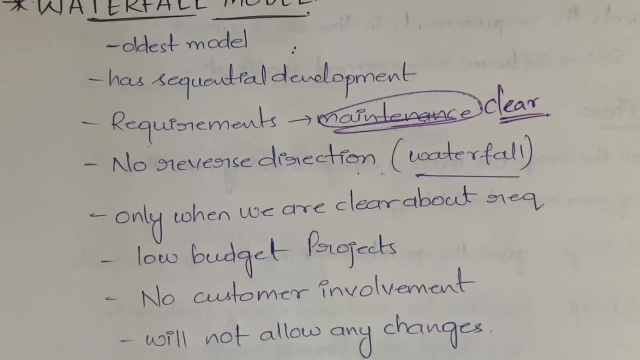 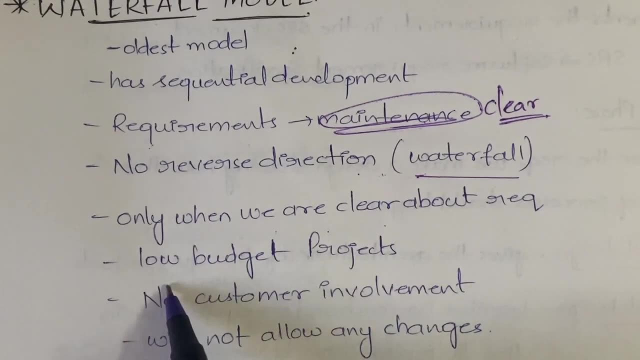 So that is exceptional cases, But in general waterfalls, in the sense they will be falling from top to bottom right, So the same flow will happen Only when we are clear about the requirements. Okay, done, Okay, okay, I understood why I have written this. Got it, got it. 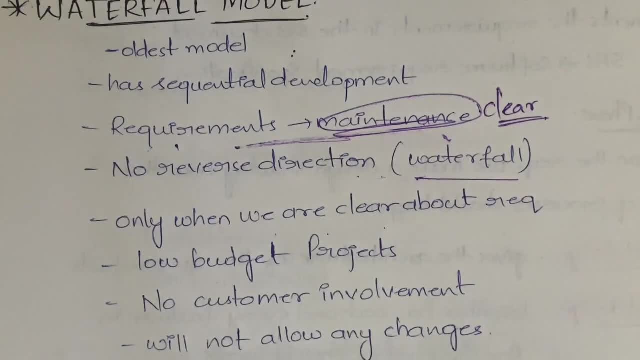 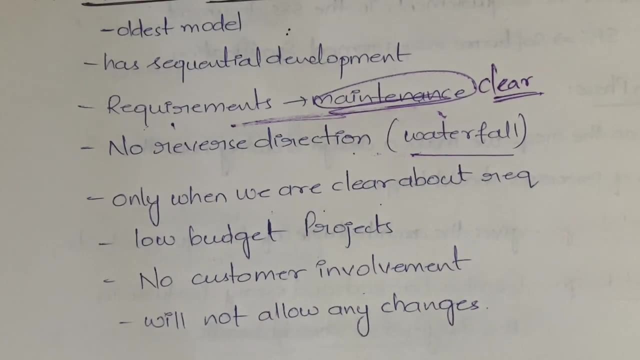 Requirements phase to maintenance phase. Now I remember I am sorry. Okay, And when you are having low budget and no customer involvement, the customer is not involving. Because if the customer is involving, then the customer will see that and he will. he may suggest some changes, right. 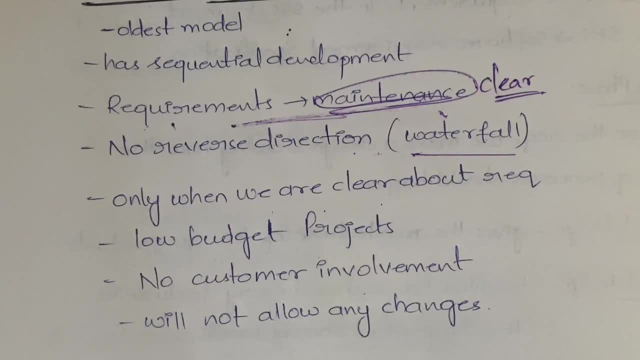 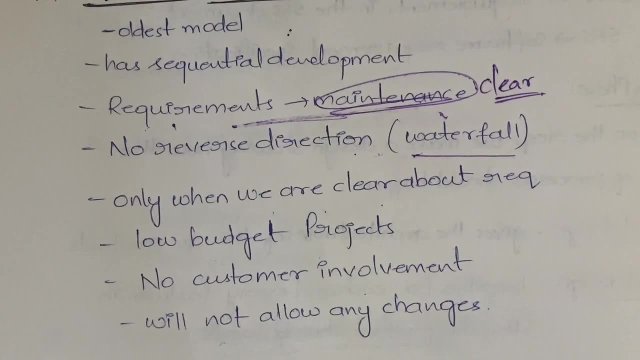 If the customer is suggesting some changes, in order to implement those changes, you have to go back to the previous step. But that is not possible here in waterfall model. Okay, Because it will not allow any changes, Got it? This is about the waterfall model, And now let us see the diagram which represents the waterfall model. 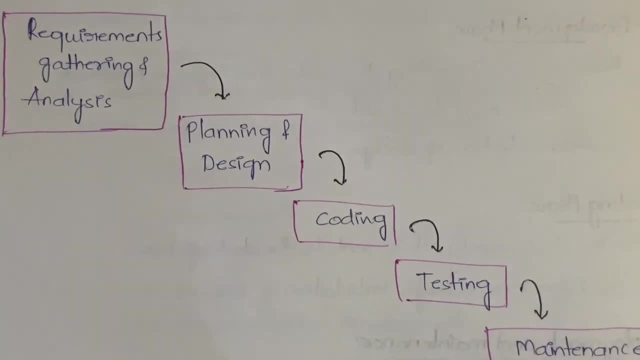 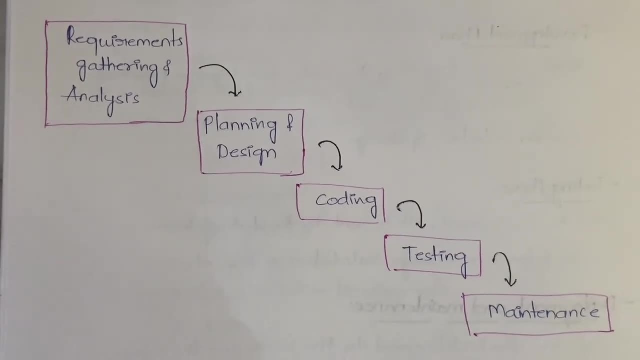 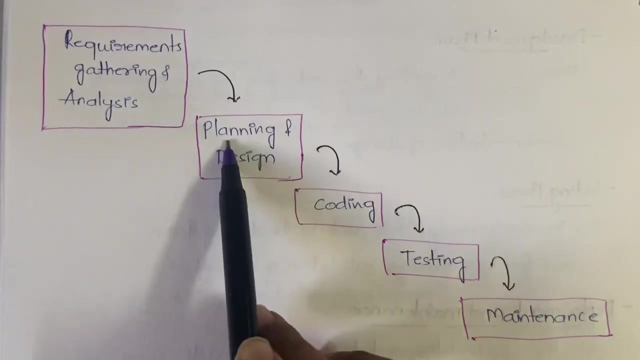 Let me zoom in a bit Some more. Yeah, So this is the diagram of waterfall model, right Starting from requirements gathering to maintenance. So in requirements gathering, what we will do in first is requirements gathering and analysis, planning and design, coding, testing, maintenance. 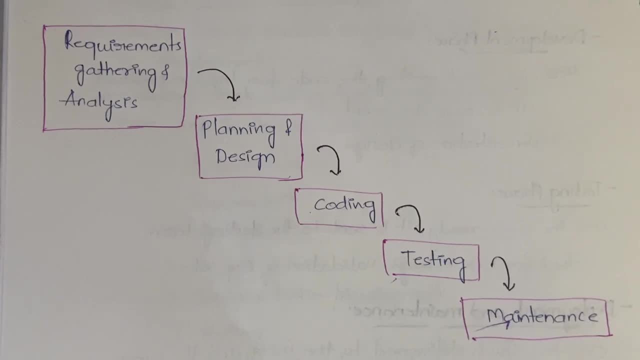 See, in this diagram we have only five stages right. But in some other website or some other video or some other textbook you may have six or you may have seven. Like SDLC also, it is not fixed design, The design changes. 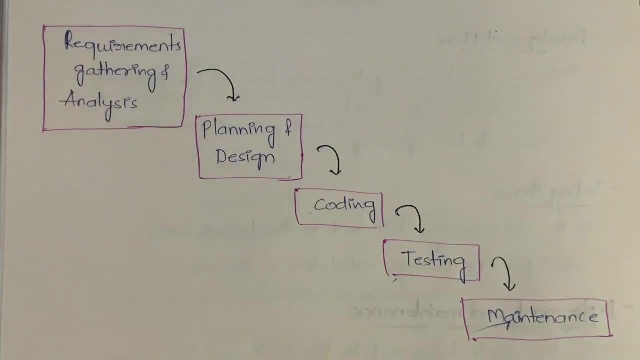 So let us see about each of them now. First phase is the requirements gathering and analysis. right, So here what happens is the basic requirements of the systems are understood. Okay, We will be understanding the basic requirements of the system and all the requirements which are related to the system which we are or the project which we are creating. you will be gathering all those requirements, Okay, Simple. 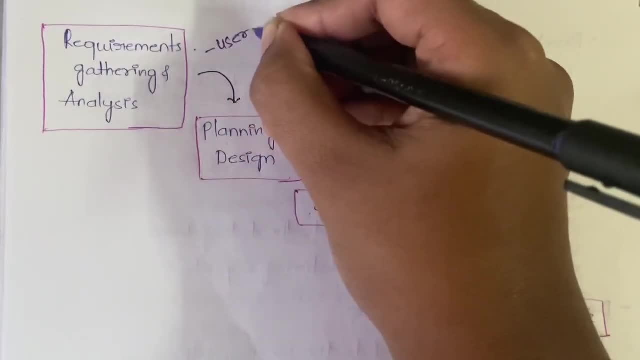 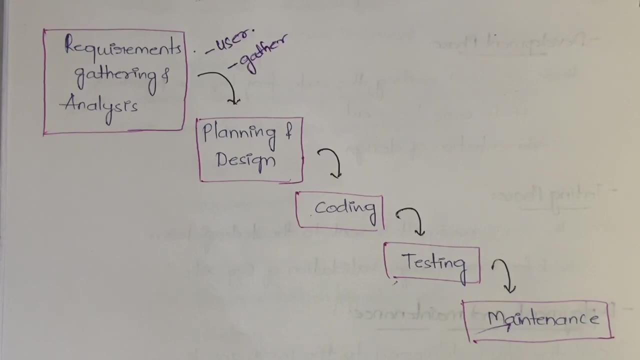 First you will get to understand the requirements from the user. Then you will gather all the requirements, That is, you will make sure you will make sure that all the requirements are there with you And then you will be documenting those requirements in the SRS document. 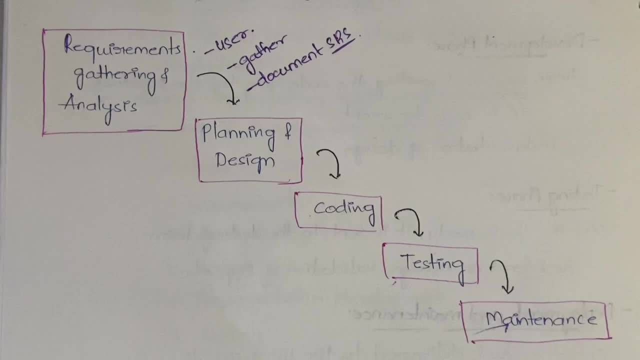 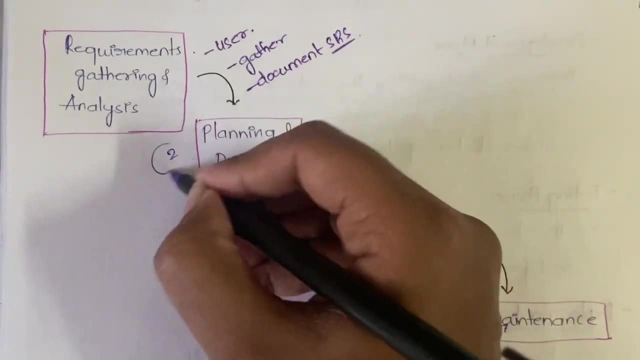 Okay, Software requirements specification document. That is what happens in the requirements gathering and analysis phase. Okay, The next phase we have is the second phase we have is the planning and design phase. So in planning and designing, what will happen is: 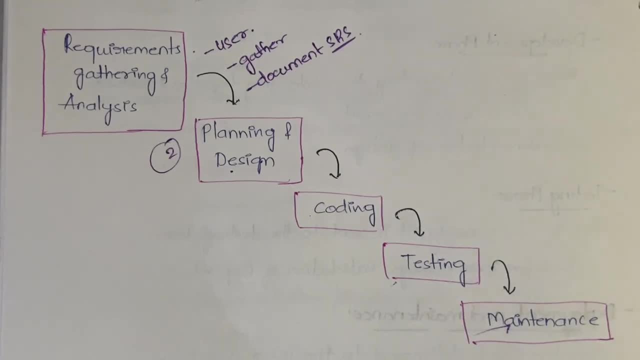 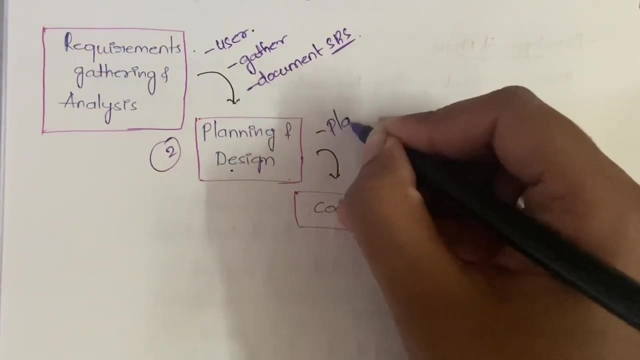 we will be planning on how to develop the software, Like how, in which stages. In first step, what we have to do. Second step, what we have to do. We will be developing a plan on how to develop the software. 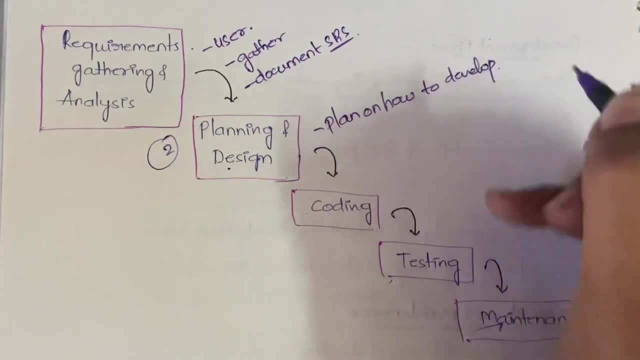 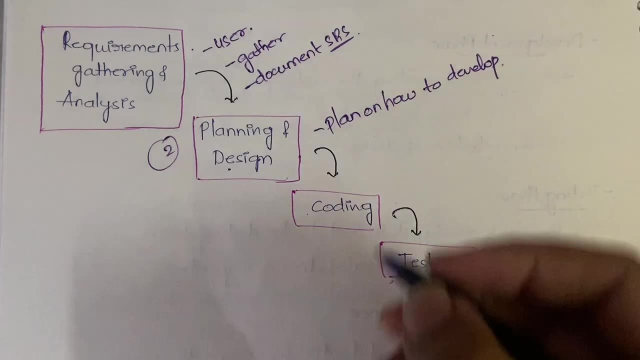 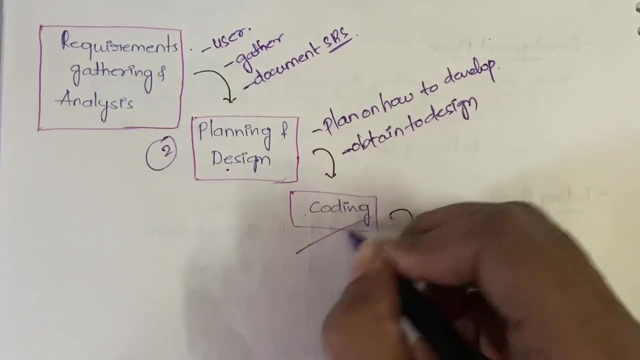 The stages, The steps. First, what we have to do. Like that, we will be developing, And next comes the design. Design in the sense you will be obtaining a design, Obtain a design. Why Design when you are doing this coding phase? 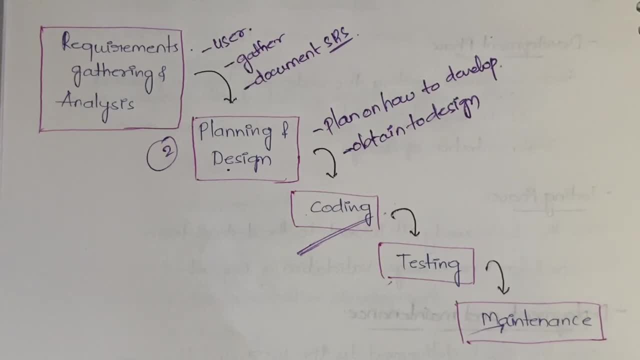 Okay, Next comes the coding. So in coding, what you will do? Simple: you will be writing the code Like code in the sense the language which a machine can understand Got it. So machine understandable format you will be converting. 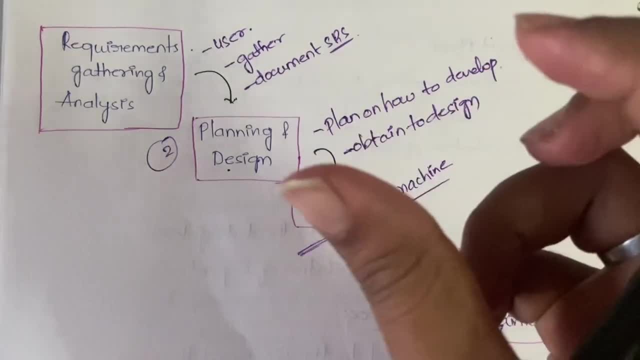 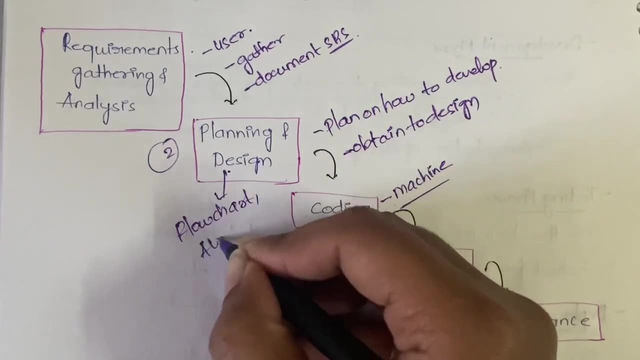 Whatever the design that you have drawn on the paper, or this design could be in any form. It can be a flow chart, Or it can be an algorithm, Or it can be a pseudo code. It can be anything, Right. 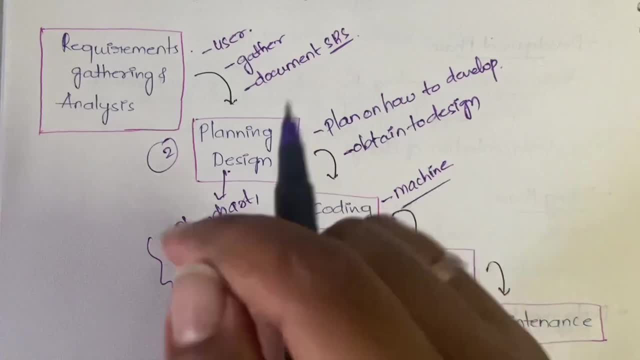 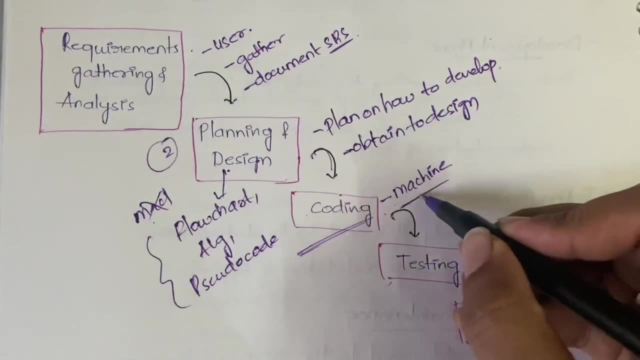 So these flow charts or algorithms or pseudo codes, whatever it is, we can understand it, But the machine cannot understand, Right? So you will be writing a code which is nothing but the language which is understandable by the machine. Got it? 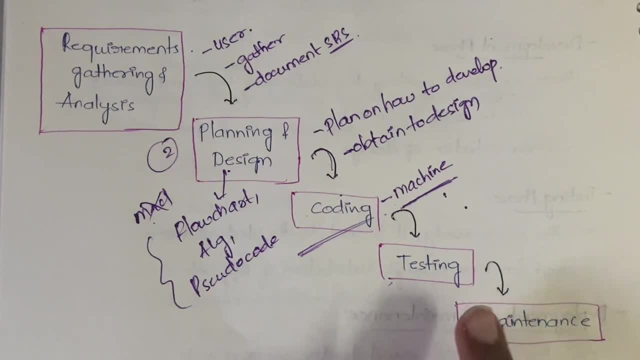 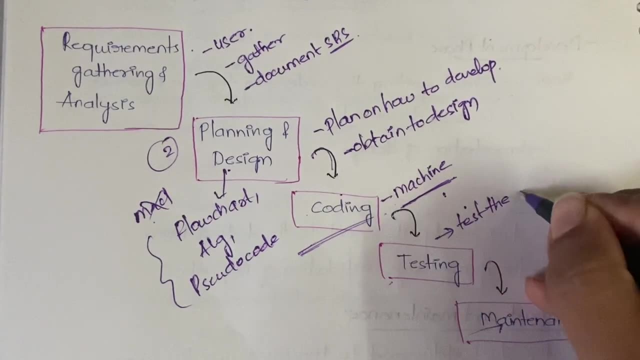 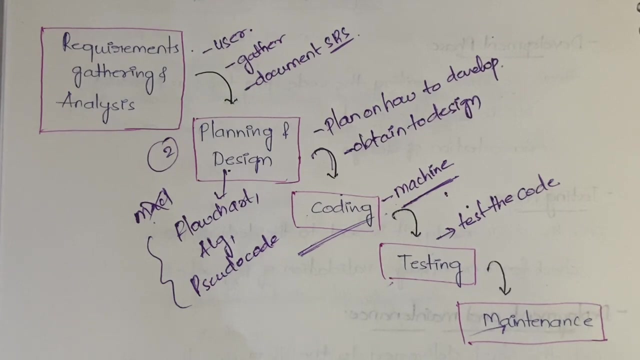 Next, After coding, what do we have Testing Here? in testing what you will do, You will test the code which you have written. Okay, The tester will do this. You will test the code. Once you are done with the testing of the code, you will find all the errors, bugs, any issues, anything wrong. 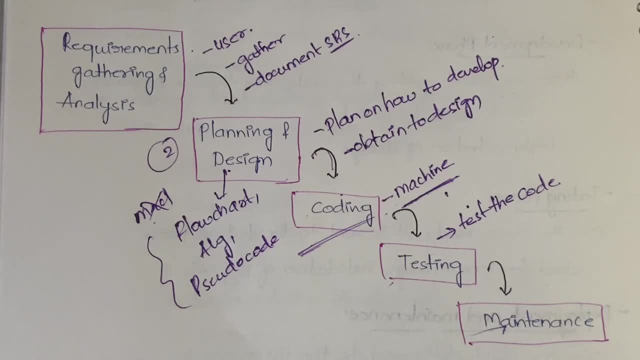 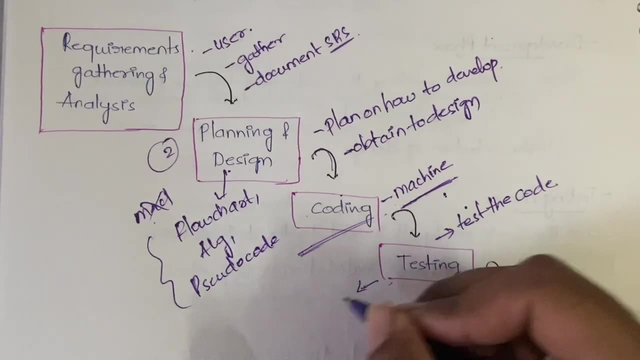 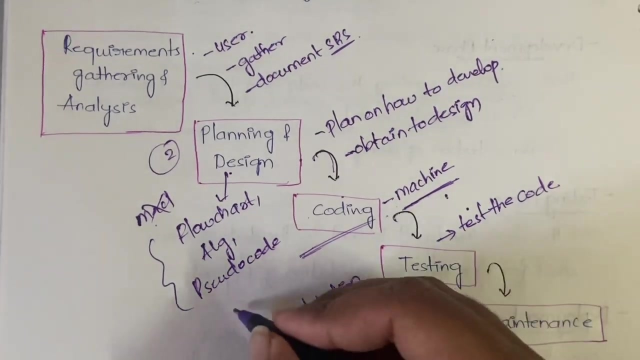 You will identify all those things And you will send to the developers team again. Developers will modify it And apart from that, in the testing, validation of requirements also will happen. What do you mean by validation of requirements? You will be having the list of the requirements given by the user. 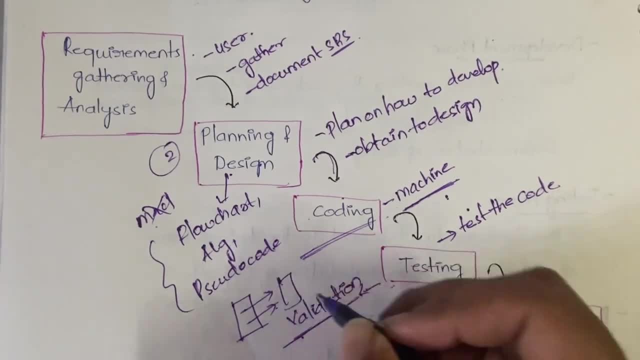 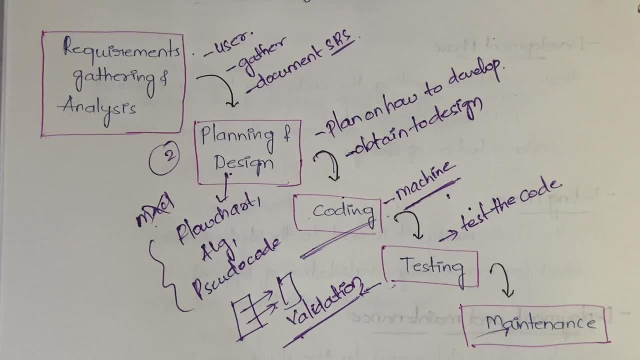 And you will be matching each of those requirements. All of those requirements are implemented or not in the project. Okay, Validation testing also will be done. Along with that, it will also focus on the logical functionality of the system, That is, whether the system is functioning properly or not. 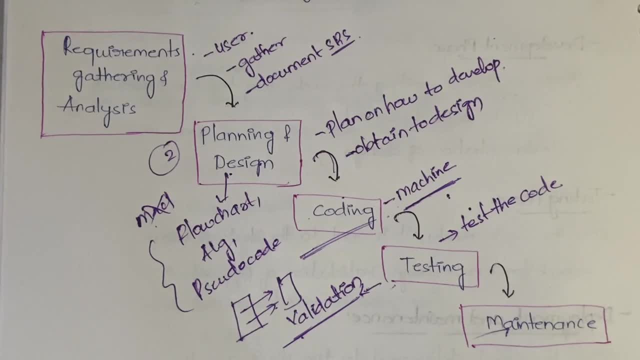 Logically, component wise, everything. Everything is working perfectly or not. That will be tested in the testing phase After testing phase. the last one is the maintenance. You already know what is maintenance. You once deploy the software to the customer. 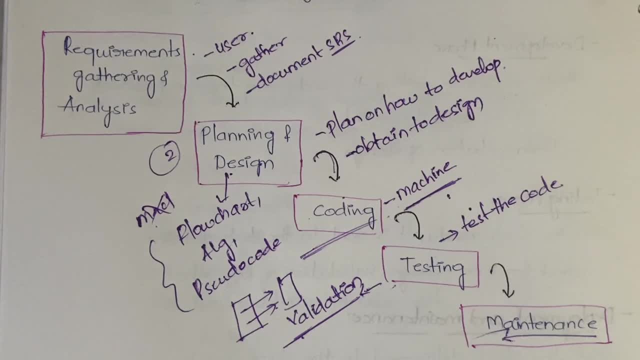 Deployment is nothing but delivering the software to the customer. Once you do that, if there is any issue or any problem to the customer, you have to go and fix that problem on time. Okay, So you can say solving or fixing problems. 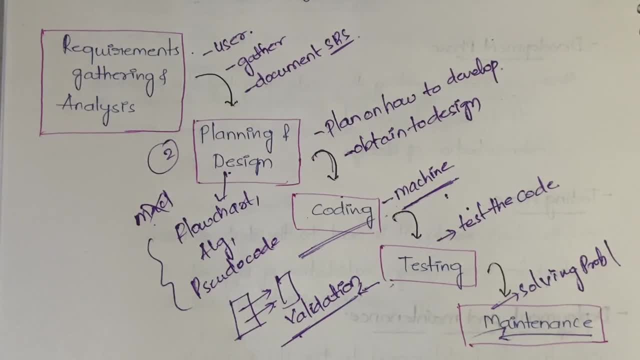 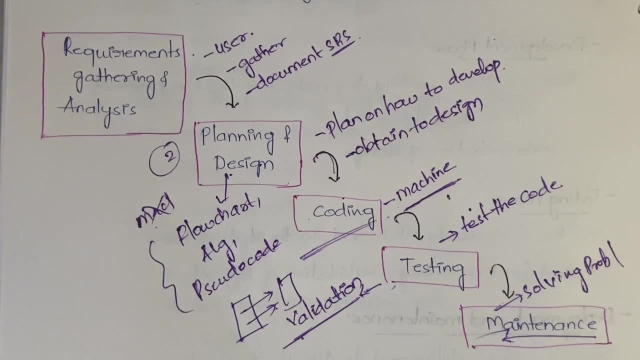 Got it. That is the maintenance. We actually have five stages in the waterfall model Requirements gathering and analysis phase, where you gather all the requirements. First, you will be collecting the requirements from the user. You will be gathering those requirements from your end. 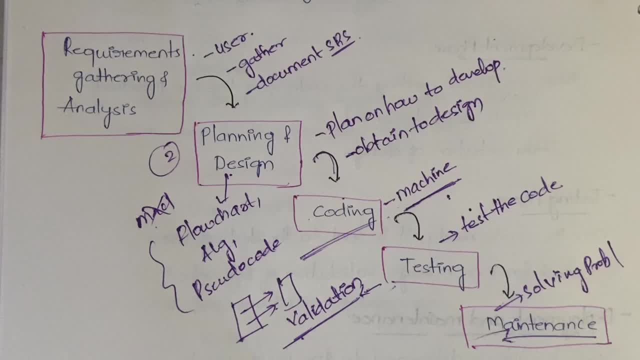 And then you will be documenting them into an SRS document. Next comes the planning and design. Here you will be establishing a plan on how to develop the software, which has all the stages and steps involved in the software, And you will also obtain the design. 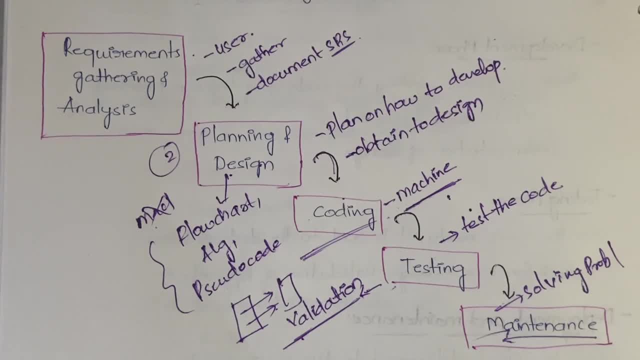 That design could be anything. It can be in form of a flow chart, It can be in the form of algorithm or anything. And next comes the coding, where you convert the design into a machine understandable form. And after coding we have testing where the requirement validations happen. 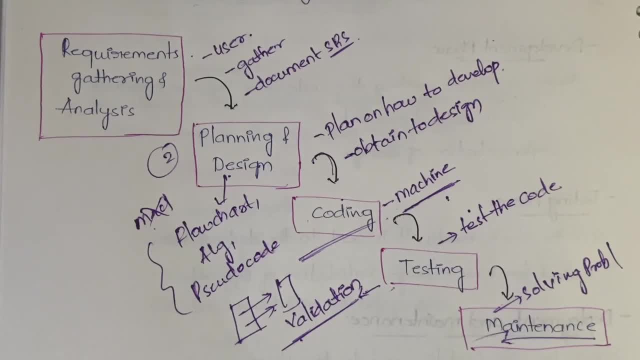 Also the code is tested. Then, after testing, if the test is successful, we move to the maintenance phase. In the maintenance phase we will be delivering the software to the customer And from there we will be taking the feedback. 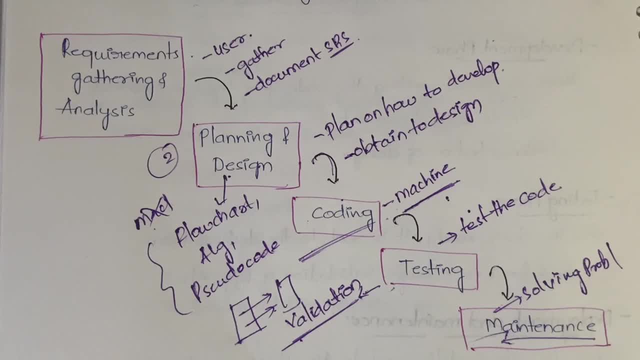 If the customer is having any issues, we will be trying to resolve them and all. And here one more thing: Software or project, or you know, there are some words which are similar. If I say software sometimes and if I say project sometimes, don't get confused.